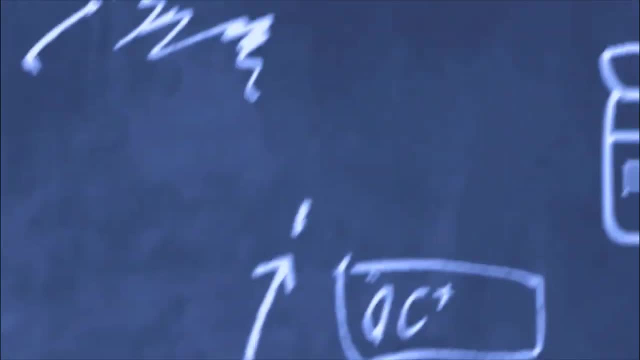 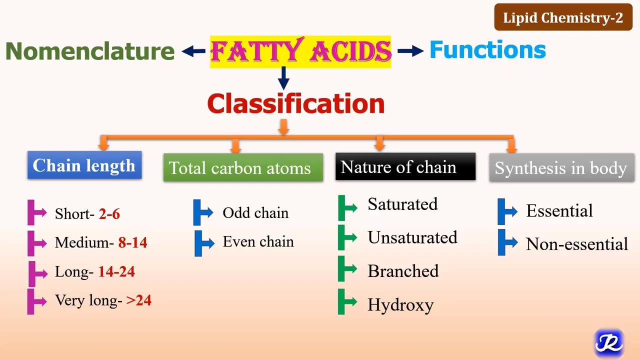 Hello everyone, today we are going to learn about fatty acids. At the end of this video, you should be able to define fatty acids, classify them with suitable examples and enumerate the functions of fatty acids. Fatty acids are carboxylic acids with hydrocarbon side. 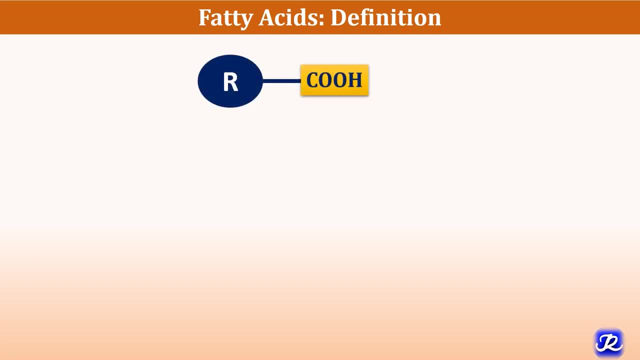 chains. They are denoted as R-COOH. R represents hydrocarbon side chain. This is the example of valeric acid. This portion represents hydrocarbon side chain and this is carboxylic acid. Hydrocarbon side chain is non-polar in nature and carboxylic acid is polar in nature. This non-polar and 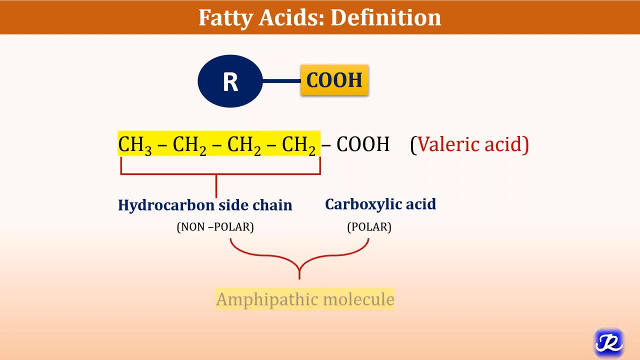 polar nature of this fatty acid make it an amphipathic molecule. In human monocarboxylic aliphatic acids are found, and these fatty acids are usually occurring in sterified form, and free fatty acids are transported in circulation bound to albumin. 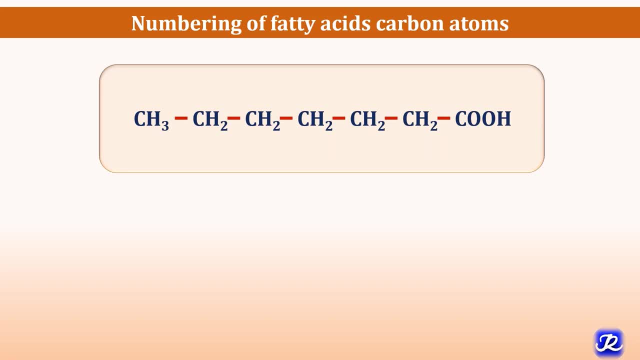 Now let's see how carboxylic acids work. Let's see how numbering of carbon atoms is done in fatty acids. This is the example of fatty acid. So the numbering of carbon atoms starts from the carboxylic acid, The carbon. 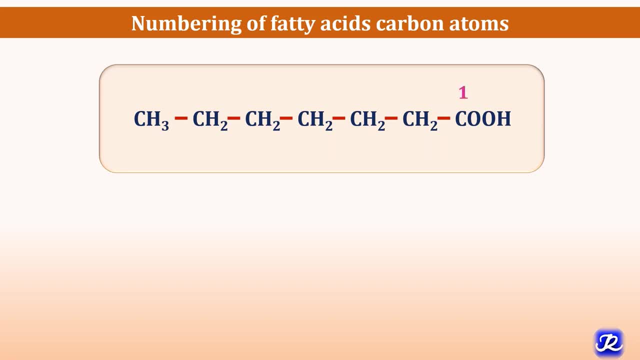 of carboxylic acid is numbered as 1.. Then this is carbon number 2,, 3,, 4,, 5,, 6 and 7.. And the second number, carbon atom, is also denoted as alpha. Third number, carbon atom is denoted as beta. 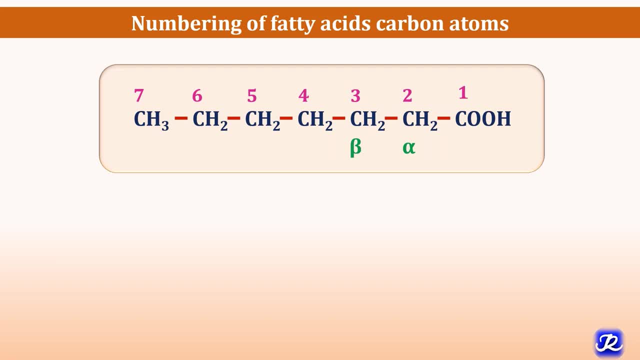 So this is the C system of numbering fatty acids. What is the omega system of numbering fatty acids? In the omega system, numbering starts from methyl N, So the carbon atom present in the methyl N is denoted as omega 1, omega 2, omega 3, omega 4, omega 5, omega 6, omega 7, omega 8, omega 9, omega 10, omega 12, omega 13,, omega 14, omega 15, omega 16, omega 16.. 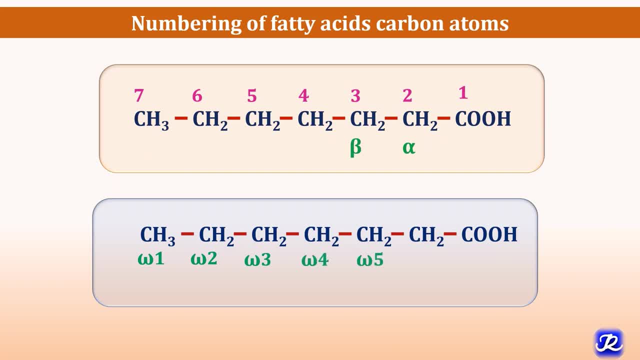 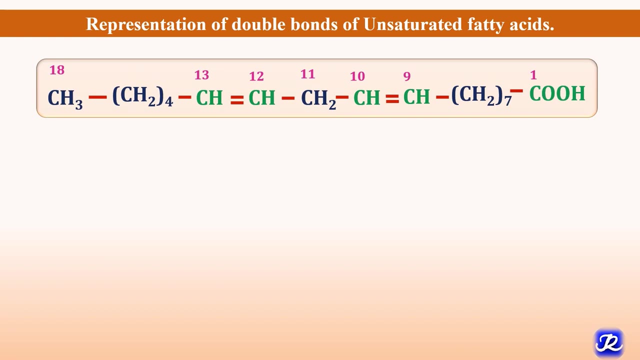 This is omega 2, this is omega 3, omega 4, omega 5 and omega 6.. This is how numbering of carbon atoms is done in fatty acids. Now let's see the representation of double bonds of unsaturated fatty acid. This is the linoleic acid, which is unsaturated fatty acid. It has 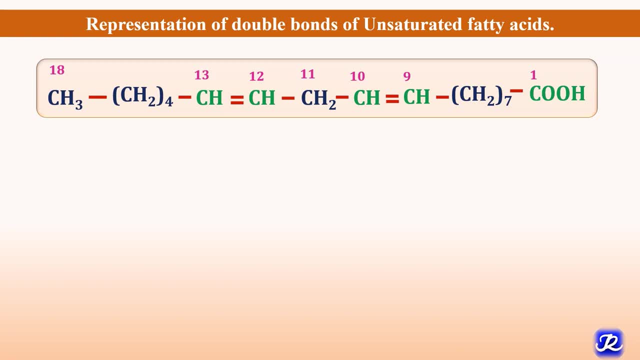 18 carbons and in the C system numbering of carbon atoms starts from the carboxy terminus. This linoleic acid is represented as C18 because total number of carbon atoms are 18.. 2 means total number of double bonds, So 2 double bonds are present in this fatty acid. 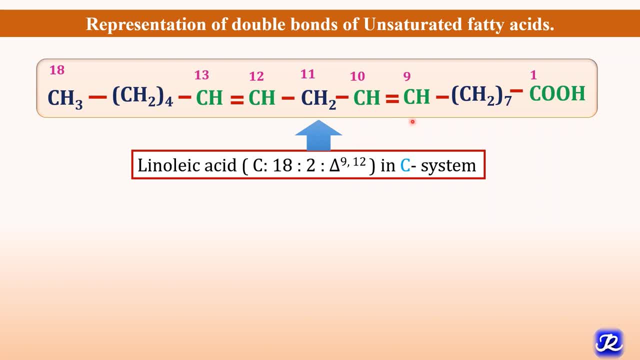 Delta 9 represents the first double bond, is between 9 and 10 and 12 represents the second double bond is present between 12 and 13.. So in the C system it is written as C18 to delta 9, 12.. 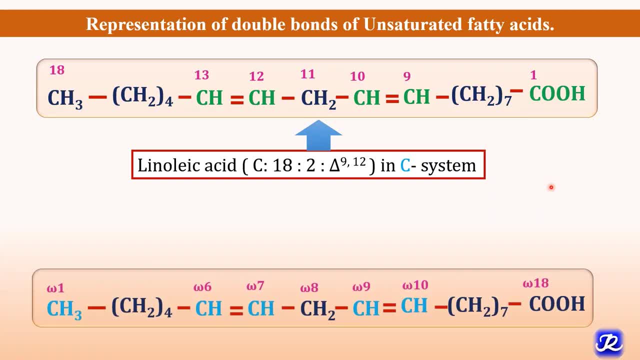 Now let's see how it is written in omega system. We know that numbering of omega carbon starts from the methylene. This is the omega 1 carbon and this is omega 18 carbon. In the omega system, linoleic acid is written as C18, as total number of carbon atoms are 18.. 2 double bonds are there. 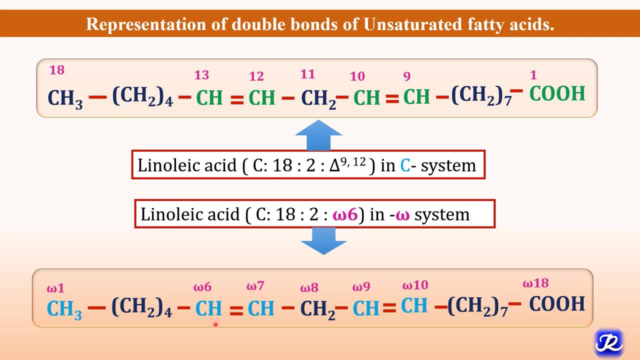 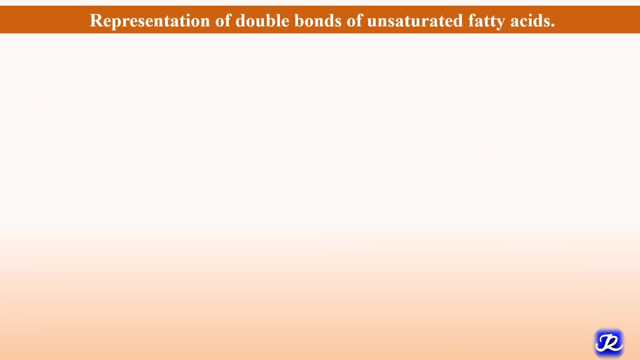 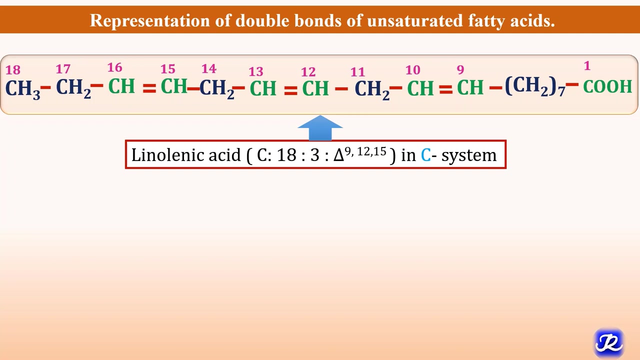 and omega 6 means the first double bond is between the carboxy terminus- So in the C system it is written as C18- to omega 6.. So linoleic acid is an example of omega 6 fatty acid. Let's take other example of linoleic acid. This linoleic acid has 18 carbons and in the C system 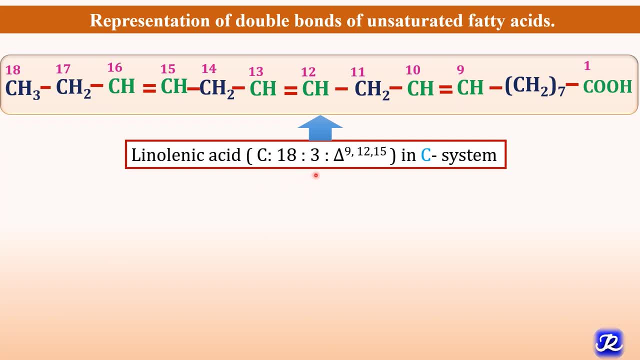 it is represented as C18,. 3, 3 denotes 3 double bonds, and delta 9 shows that it has 18 carbons. So the first double bond is present between 9 and 10,. 12 shows the second double bond is present. 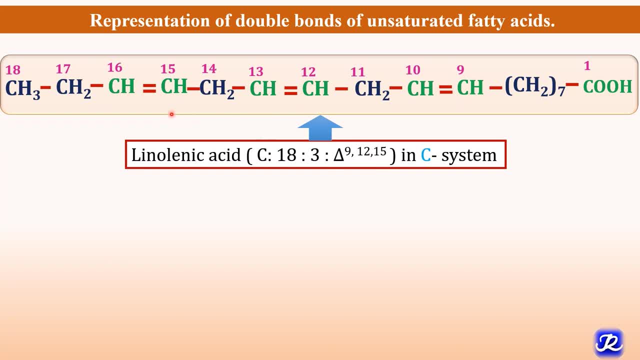 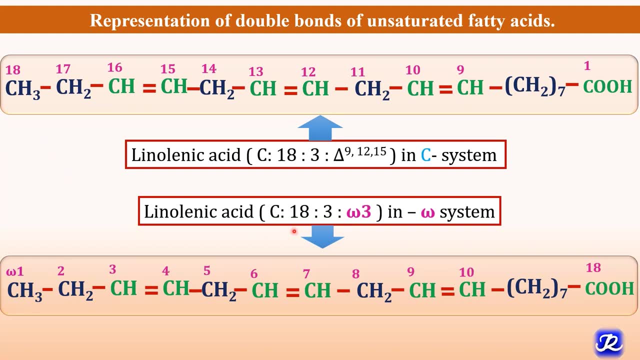 between 12 and 13, and 15 means third double bond is present between 15 and 16.. In the omega system it is written as C18, 3, omega 3.. Omega 3 means the first double bond is present between: 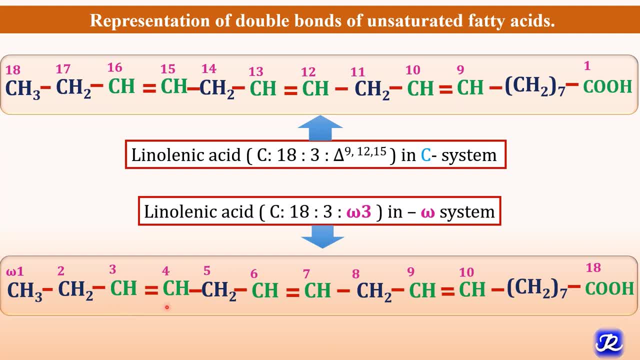 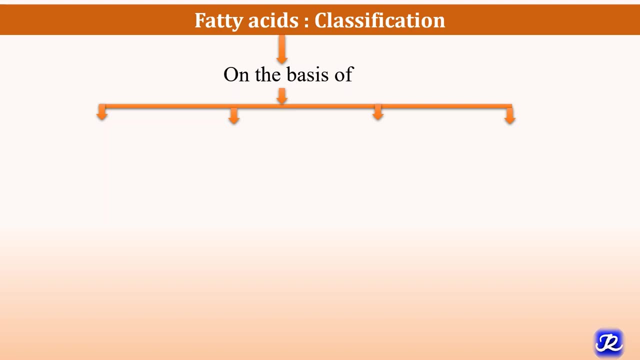 carbon, omega 3 and omega 4.. So this linoleic acid is omega, omega-3 fatty acid and this is how it is represented in the omega system. How fatty acids are classified? They are classified on the basis of chain length. 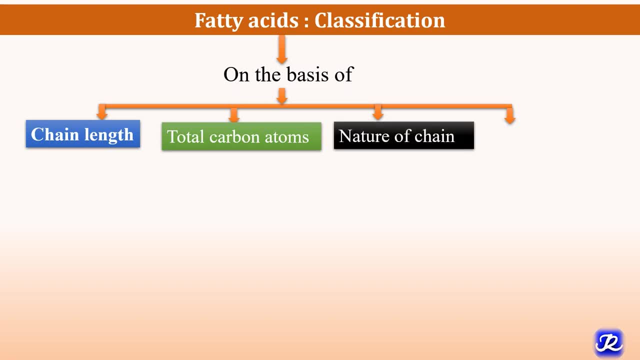 total carbon atoms, nature of the chain and whether they are synthesized in the body or not. So, depending on the chain length, they are again classified as short fatty acid if number of carbon atoms are 2 to 6, medium fatty acids if 8 to 14 carbon atoms are present. long chain if 14. 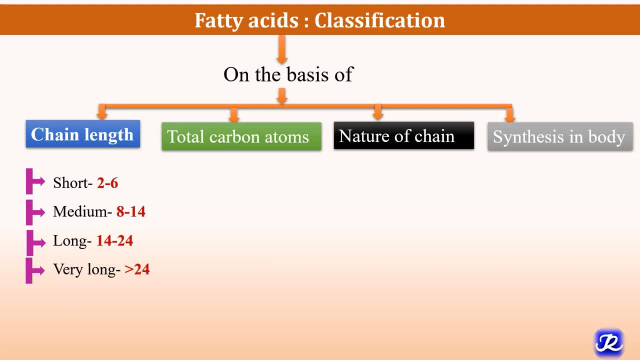 to 24 carbon atoms are present, and very long if more than 24 carbon atoms are present. We will see the examples in the later slides. Depending on the total carbon atoms, they are classified as odd chain fatty acids and even chain fatty acids. The example of odd chain fatty acids are: 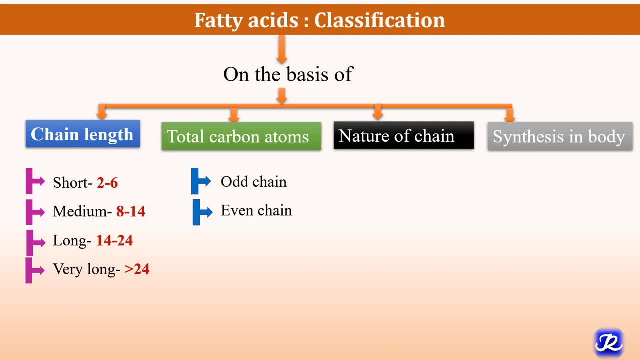 propionic acid, valeric acid and even chain fatty acids are palmitic acid, stearic acid and fatty acid. in the biological system usually contain even carbon atoms, typically between carbon 14 and 24.. Depending on the nature of chain, they are classified as saturated. 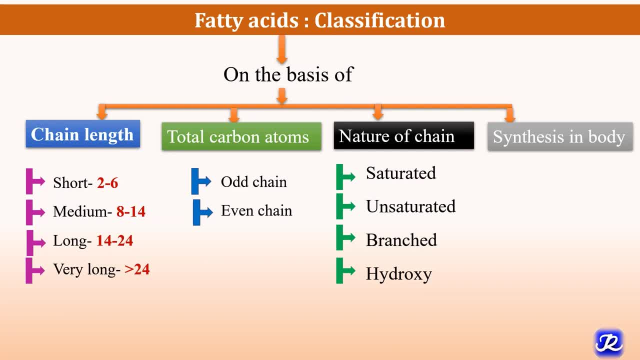 unsaturated, branched or hydroxy fatty acid. Saturated fatty acids do not contain double bond. Unsaturated fatty acid contains double bond. Branched fatty acid: the example is isovaleric acid, which is the metabolic intermediate. Hydroxy fatty acid: the example is cerebronic acid. 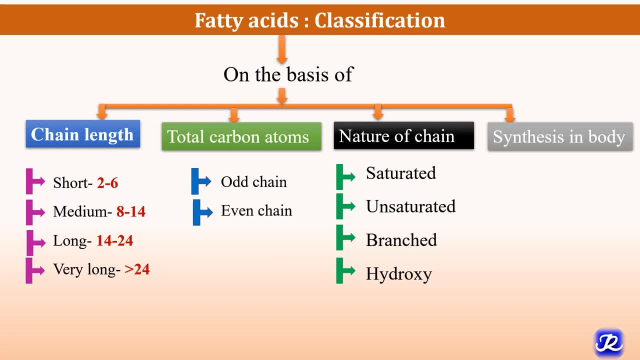 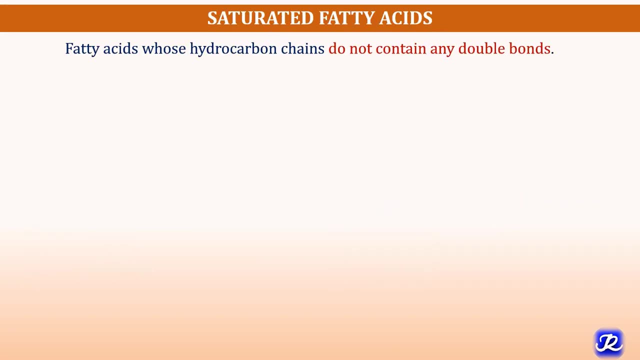 which is present in the brain. Depending on the synthesis, they are classified as short long chain fatty acids. for��i acid, Actual fatty acids are classified as essential if they are not synthesized in body and non essential are synthesized in the body. Lets see some examples and the sources of Saturated Fatty acid. Saturated fatty acids. 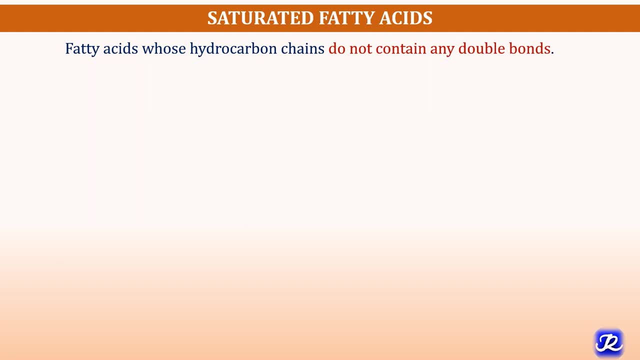 are those whose hydrocarbon chain does not contain any double bonds. They are associated with high levels of total plasma cholesterol, heavy food traces, highORT, and so on, up to 9 and until 4.0.. We are discussing exercises daily to tolerate higher levels of total plasma cholesterol. and then stop dieting. Today we will be discussing faster fasting, добрag aliment products, including Light product, eating daily and not adding diet. and besides this, we will discuss談가 polimhar therapy and今 schöne खglरों utapin42. If we are fasting regularly, what exercises should we interpret after first? 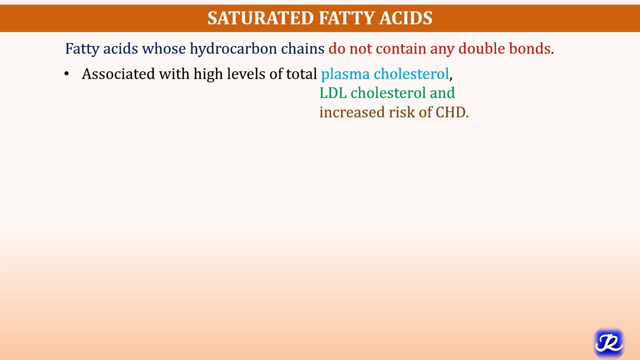 LDL cholesterol and increased risk of coronary heart disease. The various examples are: the saturated fatty acid containing two carbons is acetic acid. It is a small chain fatty acid and the source is vinegar. Butyric acid has four carbon atoms and caproic acid has six carbon atoms, and they are also called as small chain fatty acid. 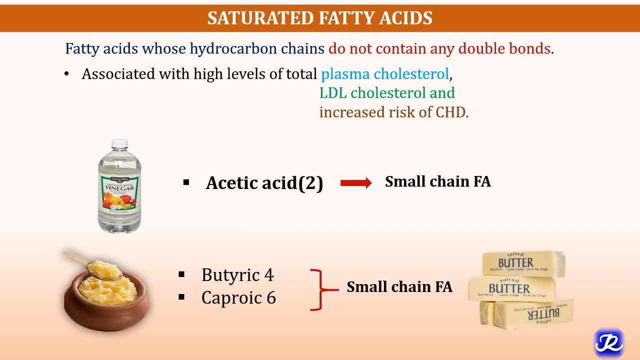 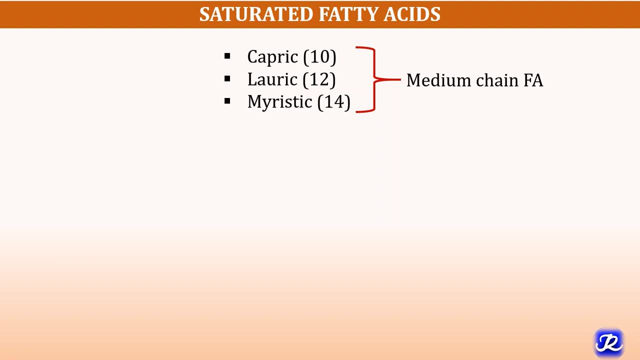 And the sources are ghee and butter. Capric acid, lauric and myristic acids are medium chain fatty acid and they contain carbon atoms 10, 12 and 14 respectively, and the source is coconut oil. Palmitic acid has 16 carbon atoms. stearic acid has 18 carbon atoms and they are long chain fatty acids. 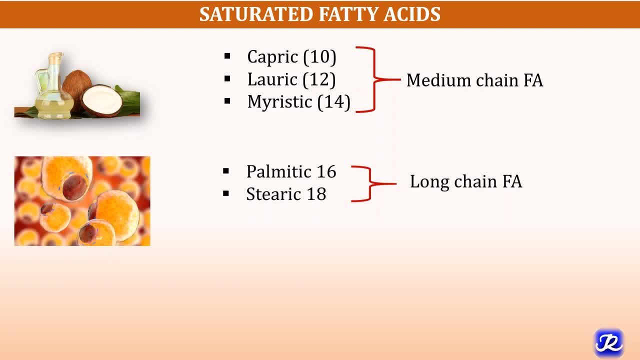 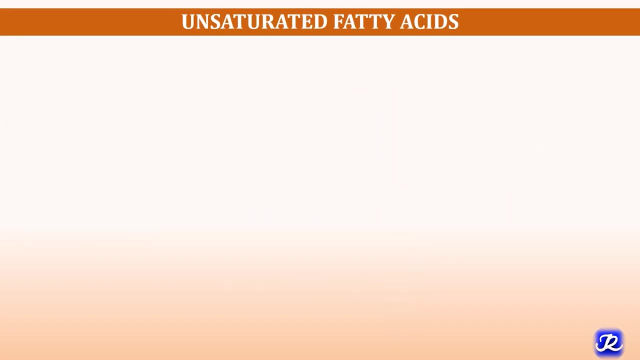 Which are present in the adipocytes. They are most potent in increasing serum cholesterol, And arachidic acid has 20 carbon atoms and it is present in peanut oil. Now let's see the examples and sources of unsaturated fatty acids. There are two types of unsaturated fatty acids. 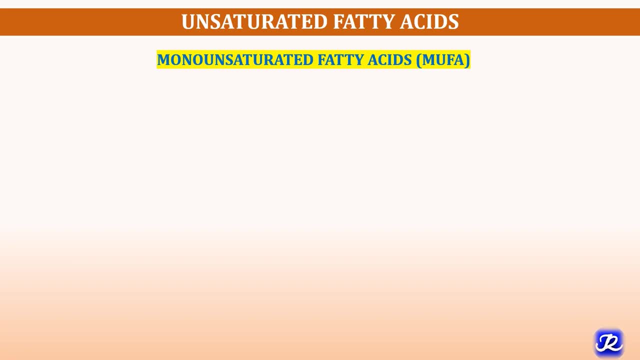 Monounsaturated, that is, MUFA, which contains one double bond, And polyunsaturated, PUFA, which contains more than one double bond. The examples are palmitoleic, oleic, erucic and nirvonic acid. Palmitoleic and oleic acids are present in adipocytes. 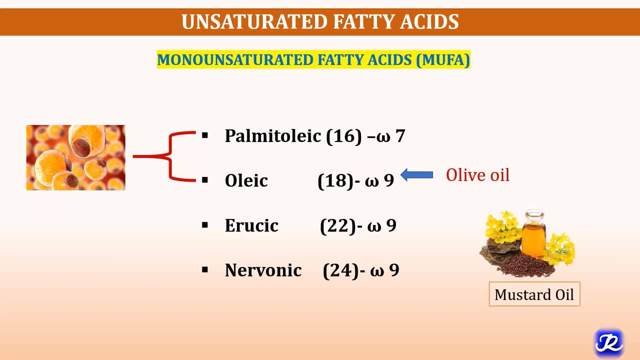 Olive oil is a rich source of oleic acid. Mustard oil is a source of erucic acid and nirvonic acid are present in brain. MUFA lower total cholesterol levels And LDL cholesterol level, but it maintain or increase HDL cholesterol. 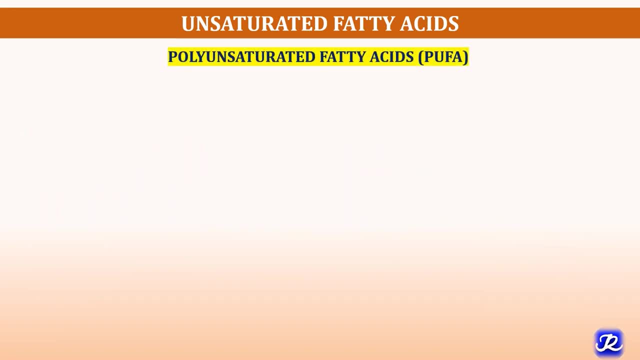 Let's see the examples of PUFA, that is, polyunsaturated fatty acid which contains more than one double bond. They are linoleic acid, which has two double bonds, and it is omega 6 fatty acid. Linolenic acid is omega 3 fatty acid. it has three double bonds. 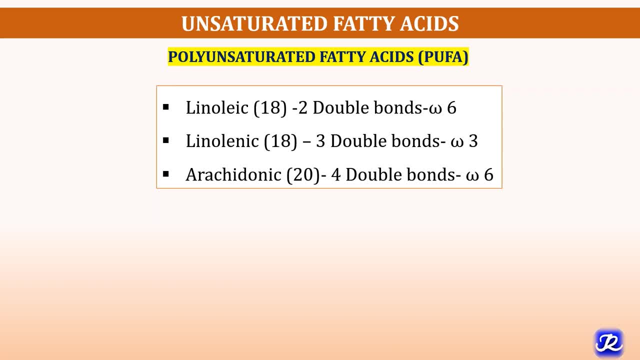 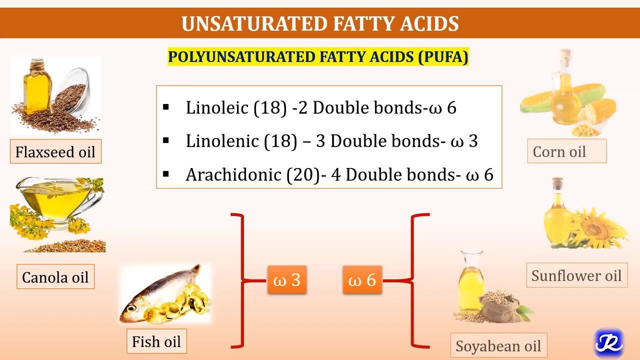 And arachidonic acid has four double bonds. It is omega 6 fatty acid. The sources of omega 3 fatty acids are fish oil, canola oil and flaxseed oil. The sources of omega 6 fatty acids are soya bean oil, sunflower oil and corn oil. 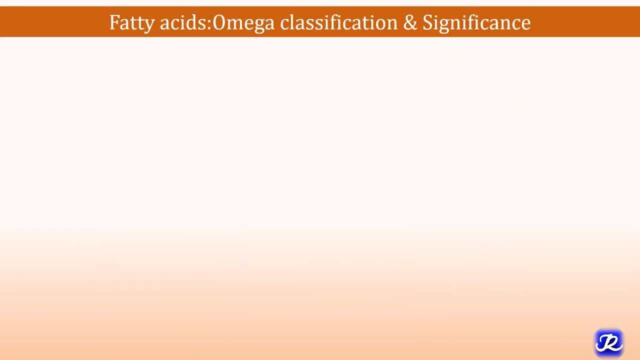 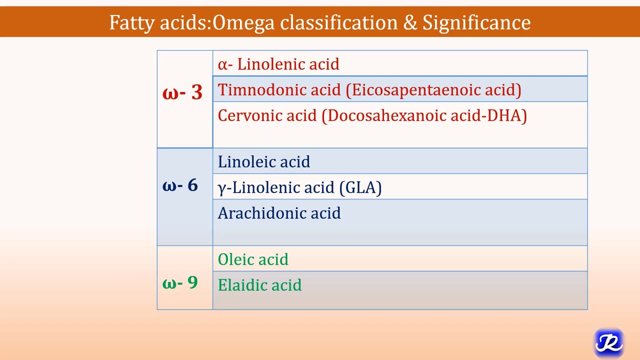 Now let's see the omega classification and significance of fatty acids. The examples of omega 3 fatty acids are alpha linoleic acid, Timnodonic acid- ie. eicosapentaenoic acid and Sarvonic acid ie. docosahexaanoic acid, ie. DHA. 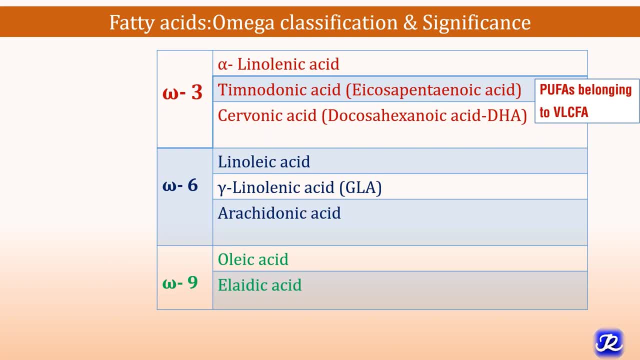 These are PUFA belonging to very long chain fatty acids, And they decrease the level of LDL cholesterol, which is bad cholesterol, Decrease the level of triacylglycerol, They decrease the platelet aggregation and thus they decrease the risk of coronary heart disease. 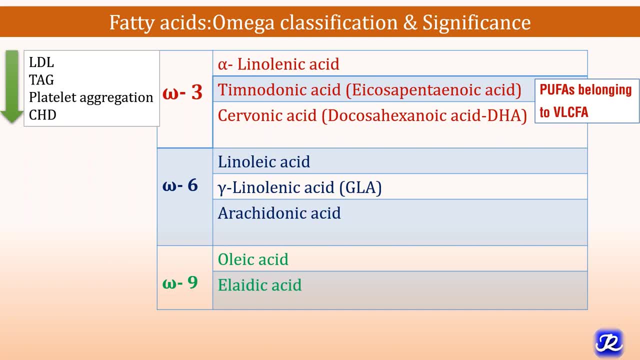 Omega 6 fatty acids are linoleic acid, Gamma linoleic acid and arachidonic acid. They are polyunsaturated fatty acids And they decrease the level of LDL, which is bad cholesterol, But they also decrease the level of HDL, which is good cholesterol. 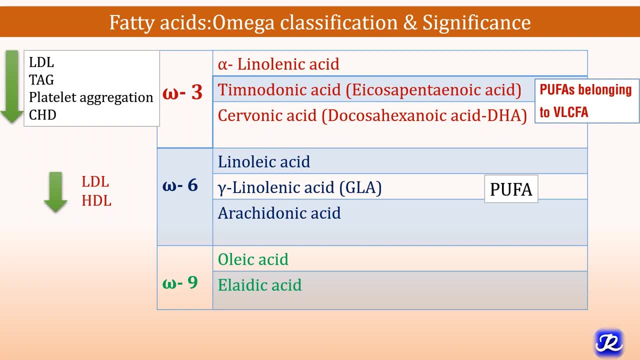 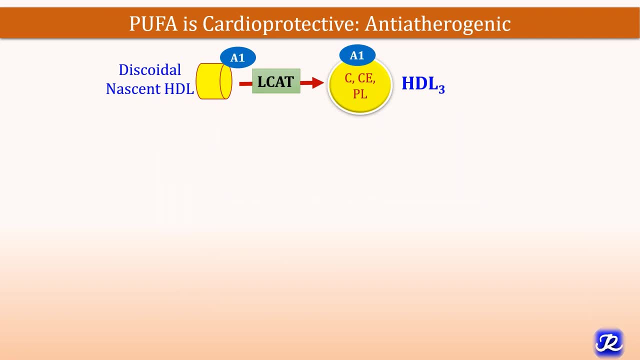 The examples of omega 9 fatty acids are oleic acid and elidic acid. They are monounsaturated fatty acids. Now let's see why PUFA is considered as cardiovascular. PUFA is anti-angioprotective, ie anti-atherogenic. 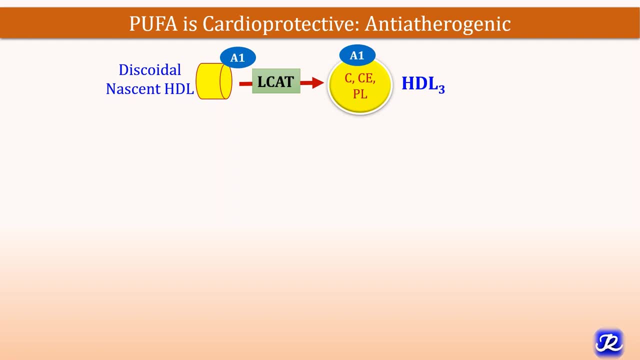 We know that the lipoprotein, HDL, ie high density lipoprotein, is considered as good cholesterol Because it transports cholesterol from peripheral tissues to liver Means. it prevents the deposition of cholesterol in peripheral tissues. One enzyme, ie LCAT, is responsible for making the discoidal nascent, HDL. 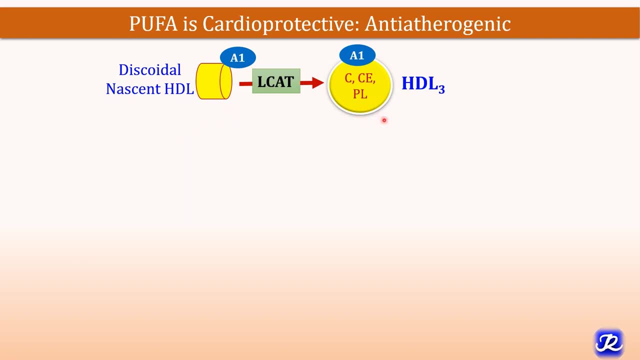 to a spherical mature HDL3.. So what is the role of this LCAT? This discoidal HDL is made up of phospholipid, mainly lecithin, And this lecithin has arachidonic acid at C2 position. 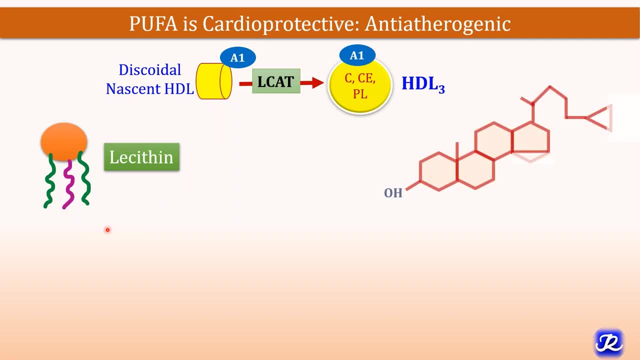 So this arachidonic acid from the lecithin is transferred to the cholesterol to form cholesterol esters And from this lecithin lysolecithin is formed. So what is the action of LCAT here? This lecithin cholesterol acyl transferase transfers the arachidonic acid from the lecithin to cholesterol to form cholesterol esters. 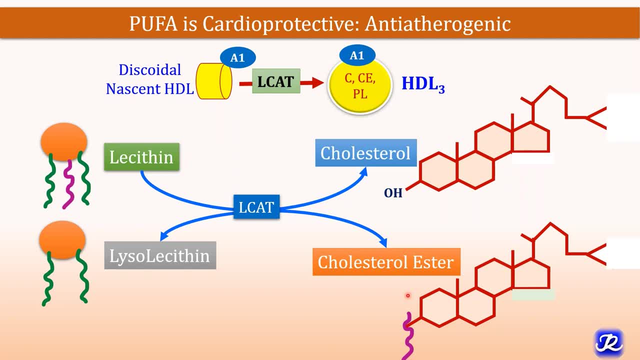 And by this esterification process the cholesterol esters move to the core of HDL molecule And it becomes spherical in size, and thus it helps in transport of cholesterol from peripheral tissues to liver By the medium of this HDL, and that's why this arachidonic acid plays a very important role in this process. 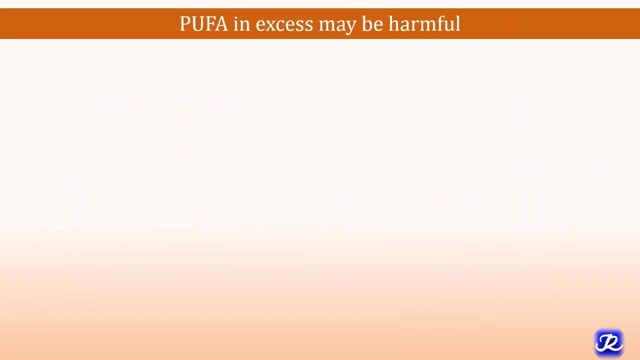 And that's why PUFA is considered as cardioproductive. Polyunsaturated fatty acid in excess may be harmful. Very high intake of omega 6 fatty acids lower the HDL level, elevate triacylglycerol level and promote platelet aggregation. 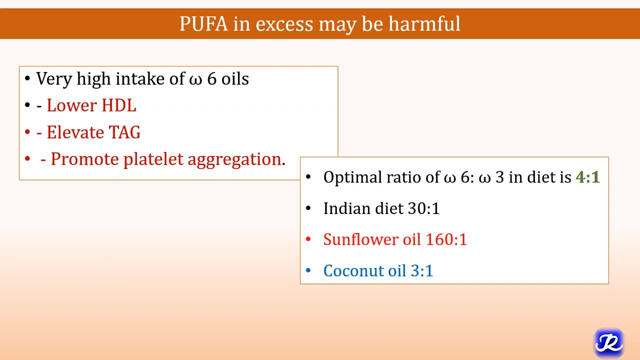 Optimal ratio of omega 6 to omega 3 in the diet should be 4 is to 1.. But Indian diet has the ratio of 30 is to 1.. Sunflower oil has the ratio of 160 is to 1 and coconut oil has the ratio of 3 is to 1.. 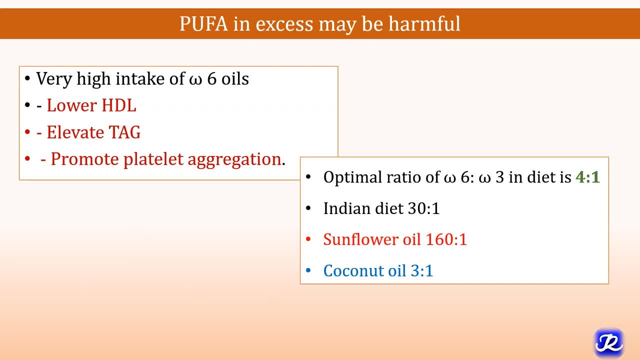 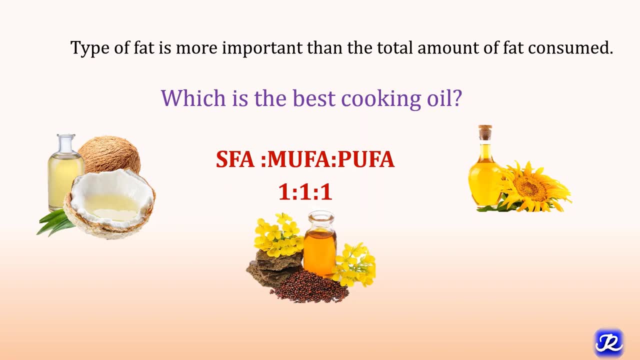 So the coconut oil in this sense, is better than sunflower oil. Type of fat is more important than the total amount of fat that is consumed. Which is the best cooking oil? As such, there is no best cooking oil. We should have equal proportion of all fatty acids, that is, saturated fatty acids. 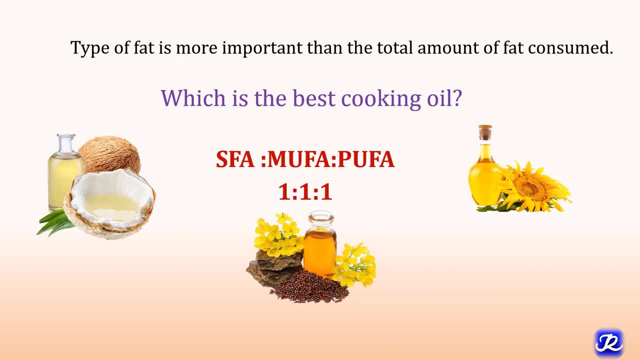 monounsaturated fatty acids and polyunsaturated fatty acids in the ratio of 1 is to 1 is to 1.. The examples that we should consume in our diet: saturated fatty acid: palm oil, coconut oil, ghee, monounsaturated fatty acid. 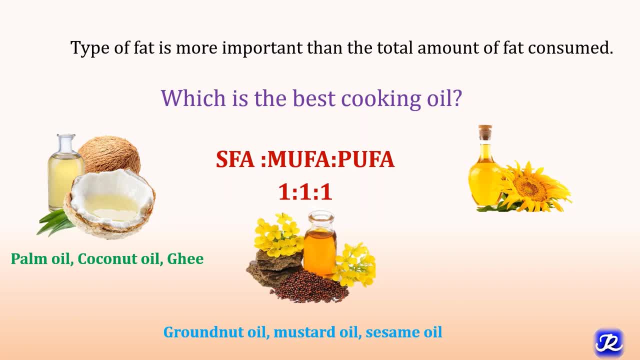 groundnut oil, mustard oil, sesame oil, polyunsaturated fatty acids, sunflower oil, rice bran oil, soya bean, corn oil. So we should have the equal proportion of all these oils in our diet. in this proportion of 1 is to 1 is to 1..